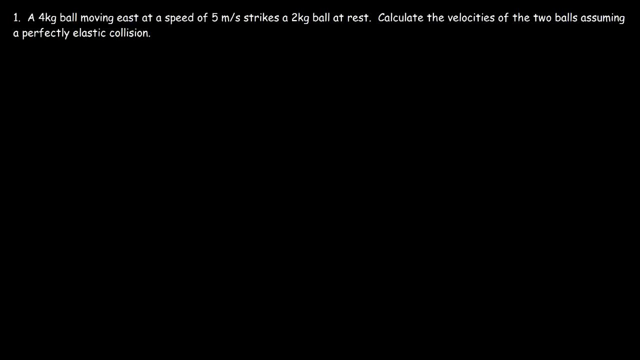 go ahead and pause the video. So what equations do we need? Now notice that we need to calculate the velocity of the first ball and the second ball, So we have two missing variables. Therefore, we need two equations. If you only have one missing variable, you need to use the conservation. 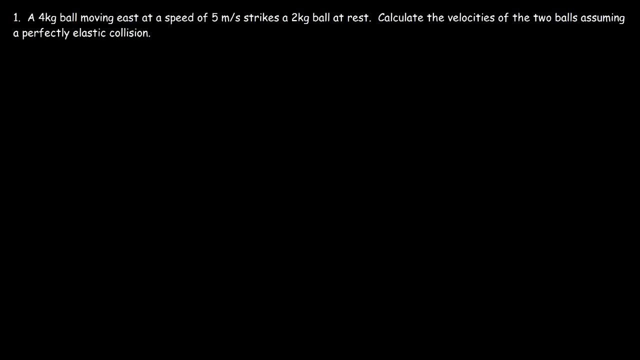 of momentum. For any collision, be it inelastic or elastic, momentum is always conserved. So m1 v1 plus m2 v2 is equal to m1 v1 prime plus m2 v2 prime. So v1 is the initial velocity of the first ball. 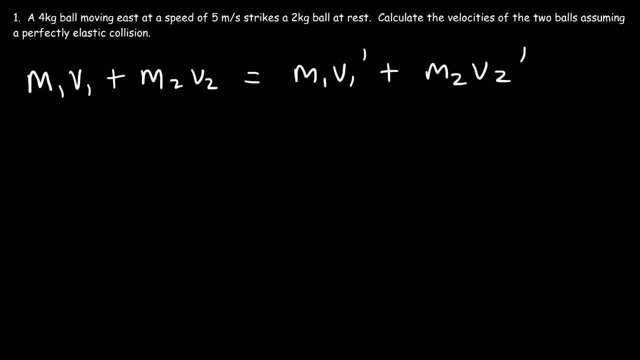 v1- prime is the final velocity of the first ball, v2 is the initial velocity of the second ball and v2- prime is the final velocity of the second ball. So what this equation is saying is that the total momentum before the collision, that is, the momentum of the first ball, is the final velocity of the second ball. 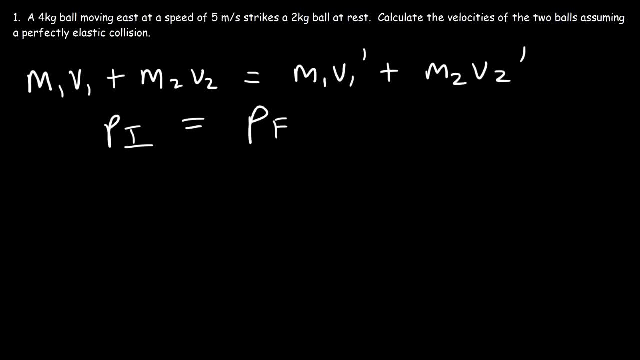 So the total momentum of both objects is equal to the final momentum after the collision. Now if you have just one missing variable, this equation will be enough to solve for the missing variable. But in this problem we have two missing variables, And so we need to use a. 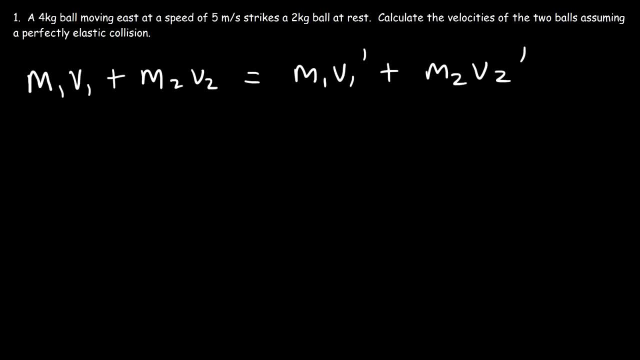 second equation: For an elastic collision, kinetic energy is also conserved. However, it is not conserved for an inelastic collision, But it's always conserved for an inelastic collision. It always has to serve for a perfectly elastic collision. 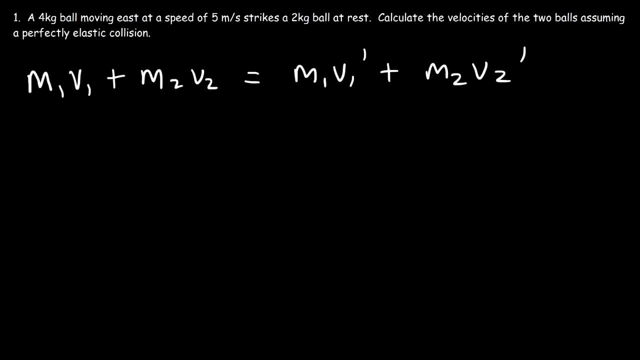 Now you don't want to use the kinetic energy formula because it's going to be a lot of work. Instead, you want to use the simplified version of the conservation of kinetic energy For these problems. that equation simplifies to this. It's the 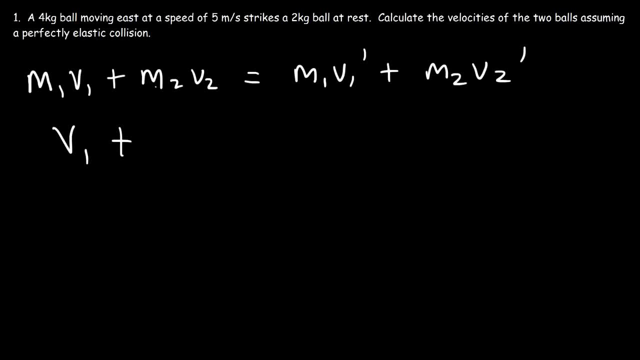 velocity of the first ball. that is the initial velocity of the first ball plus the final velocity of the first ball, And that's equal to the initial velocity of the second ball plus the final velocity of the second ball. So for elastic collisions, these are the two equations that you want to use if you need. 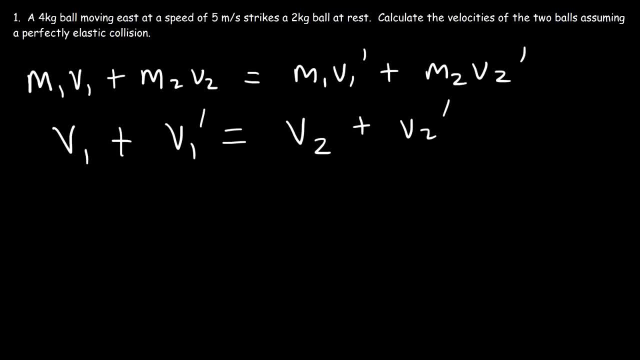 to find two missing variables. So let's start with the first equation. So we have a four kilogram ball moving east, So M1 is four, And it's moving east at a speed of five meters per second, So the velocity is positive five. 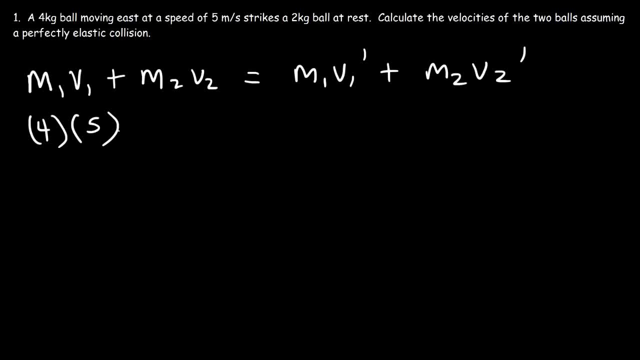 If it was moving west, the velocity would be negative and you've got to put in that negative value, Otherwise you won't get the right answer. Now the second ball is at rest. So V2 is zero, which means two times zero is going to be zero. 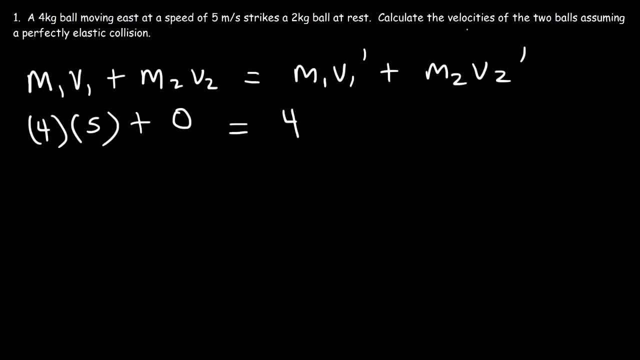 Now, the mass of the first ball is four. Now we don't know the final velocity of the first ball after the collision. That's what we're looking for. Okay, M2, the second mass or the mass of the second ball, that's two kilograms. 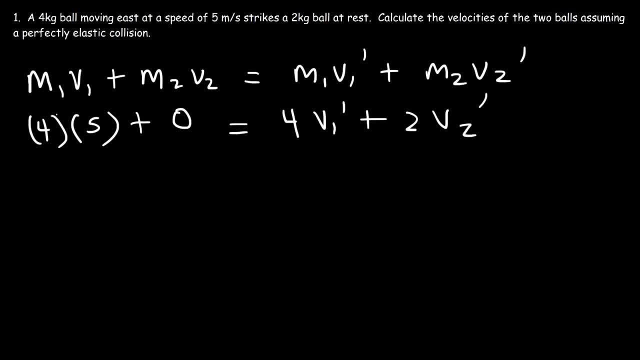 And we don't know the final velocity of the second ball. So four times five is twenty, And that's equal to four V1 prime plus two V2 prime. So let's save this equation. Now let's focus on the second equation. 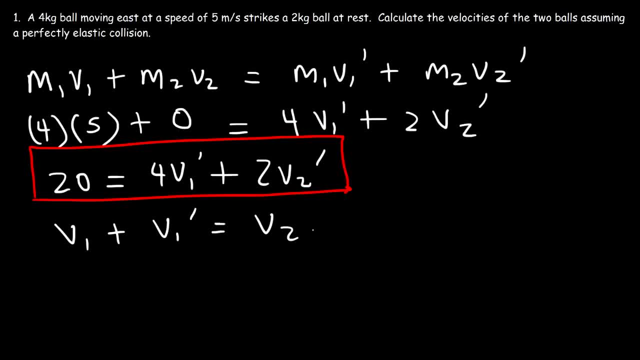 V1 plus V1 prime is equal to V2 plus V2 prime. So V1 is still five. that's the velocity of the first ball. V1 prime. we don't know what that is V2,. the initial velocity of the second ball is zero and we don't know what V2 prime is. 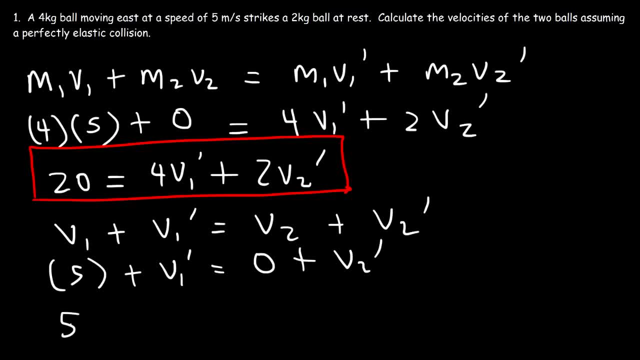 So I'm going to take this term and move it to this side. So five is equal to negative V1 prime plus V2 prime. Okay, So that's the first equation, Okay. So what I'm going to do now is line up these two equations. 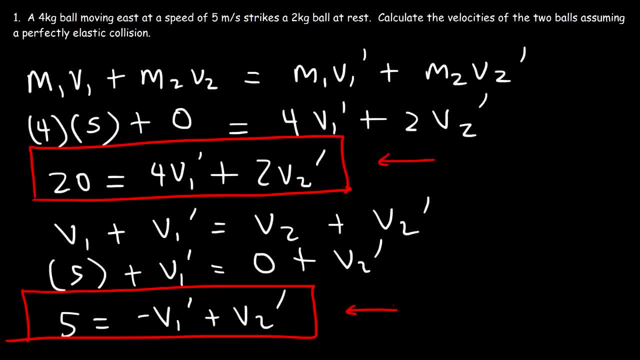 We need to solve for V1 prime and V2 prime using a system of equations. So this is going to be four: V1 prime plus two V2 prime is equal to twenty and negative V1 prime plus V2 prime is equal to five. 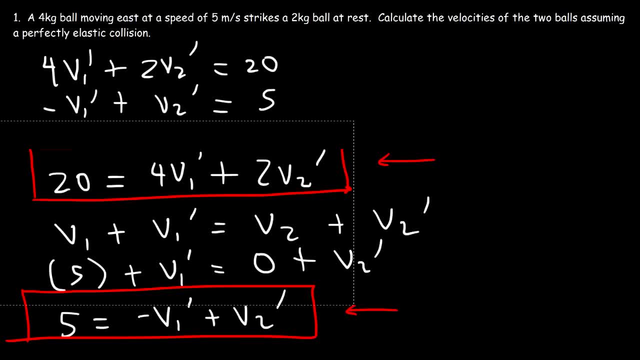 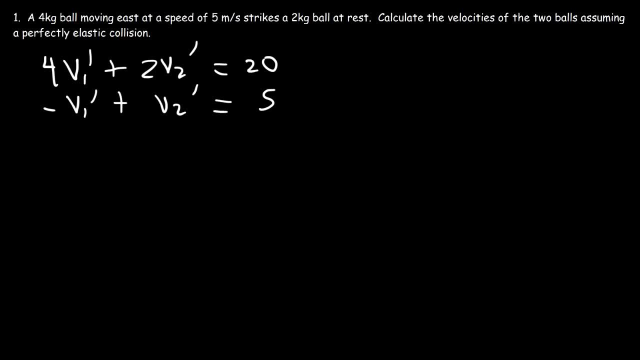 Okay, So now what we have is an algebra problem. How can we solve this system of equations? So we need to use elimination. So we have positive four V1 prime. What I need is negative four V1 prime, so that those two will cancel. 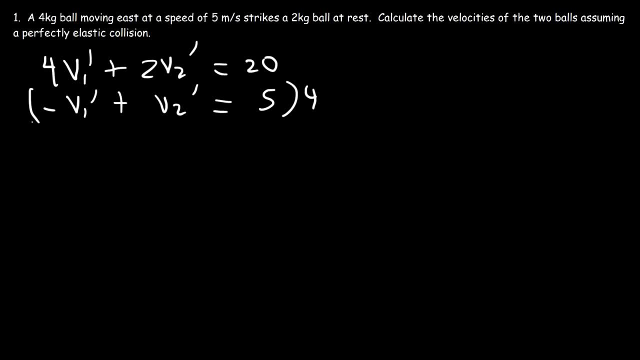 So I'm going to multiply the second equation by four. So I'm going to rewrite the first equation- Okay, It's still the same, It doesn't change. And the second equation is going to be negative: four V1 prime plus four V2 prime and five. 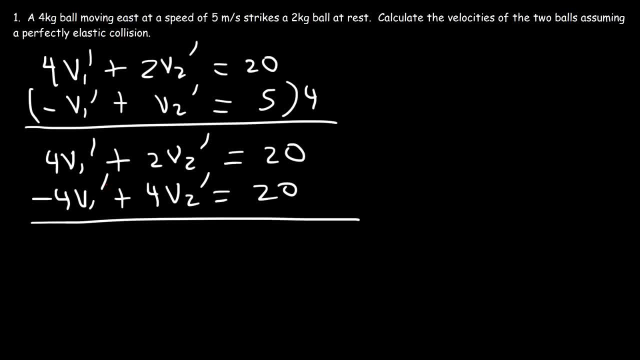 times four is twenty. So now let's add these two equations: Four and negative. four adds up to zero. Two plus four is six, and twenty plus twenty is forty. So now what we need to do is take forty and divide it by six. 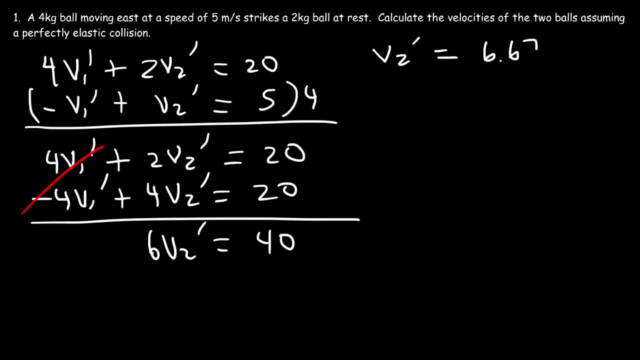 So V2 prime is 6.6.. Okay, So that's going to be 6.67 meters per second, Because it's positive. that tells us that the second ball is moving to the right with that speed. So now let's calculate V1 prime using this equation. 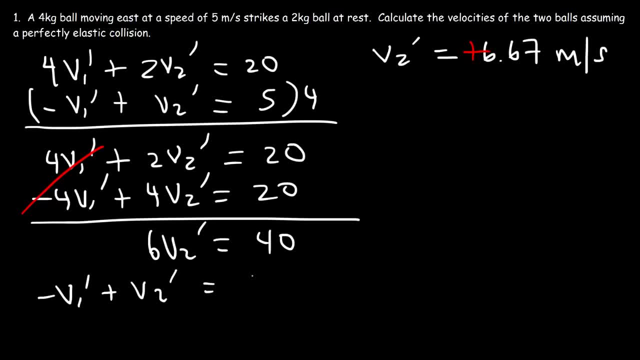 So if negative V1 prime plus V2 prime is equal to five, what I'm going to do is take this, move it to this side. so it's going to be V1 prime but positive, I'm going to take this number and move it to that side. 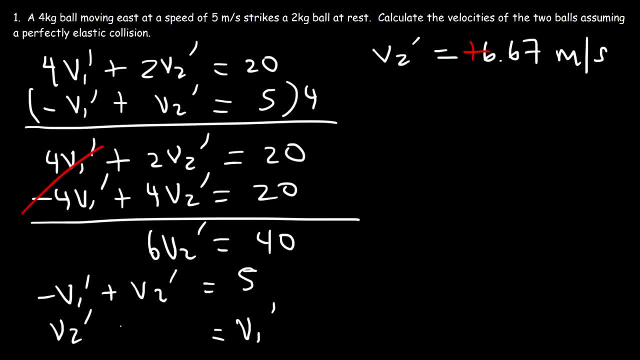 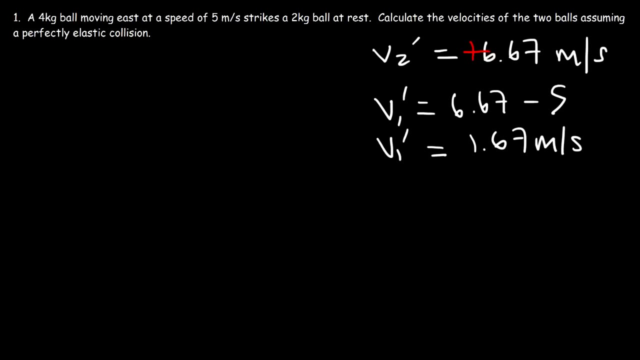 So it's going to turn to negative five. So it's V2 prime minus five. So V1 prime is going to be V2 prime, which is 6.67 minus five. So that's 1.67 meters per second. 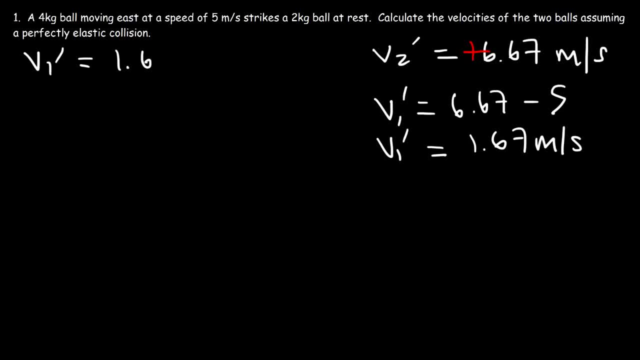 So, for the sake of space, I'm going to rewrite it here. Okay, So it's going to be V1 prime plus V2 prime plus V2 prime. Now, how do we know if we have the right answer? Well, we need to make sure that momentum and kinetic energy are conserved in this problem. 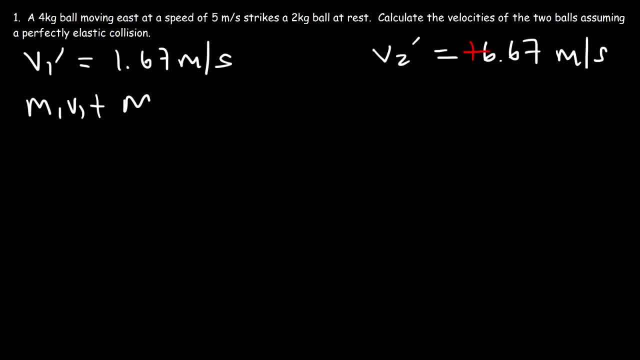 So let's start with momentum. M1 V1 plus M2 V2 has to equal M1 V1 prime plus M2 V2 prime. So the mass of the first ball is four. It has a velocity of positive five. The second ball is at rest. 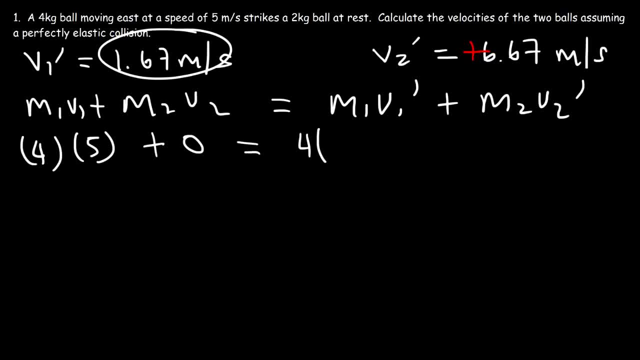 The mass of the first ball is still four, but its final velocity is 1.67.. And the second ball has a mass of two with a final velocity of 6.67.. Now, four times five is 20.. And four times 1.67 is 6.68.. 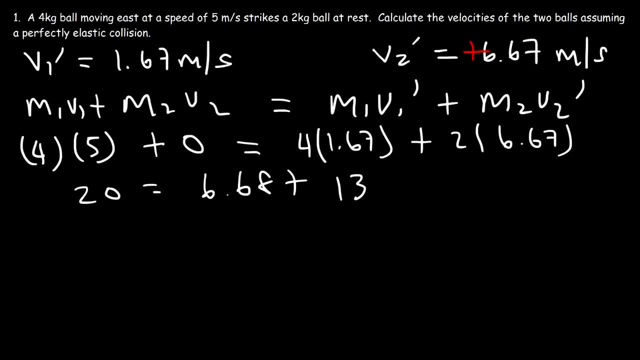 And two times 6.67 is 4.67.. Okay, So that's 13.34.. Now, if we add 13.34 with 6.68, that's going to be about 20.02, which is approximately. 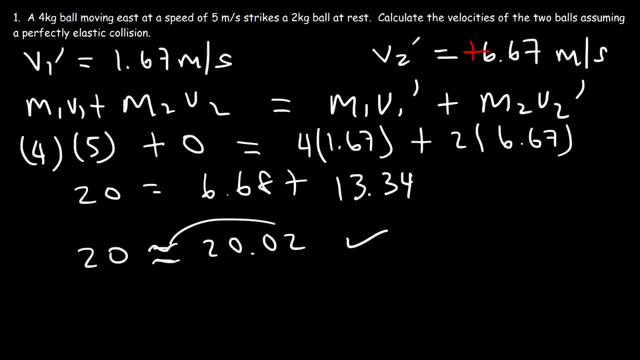 equal to 20.. So that's good enough. There's going to be some rounding error, but if it's close enough, then you know you did it correctly. So momentum has been conserved. That's a good sign. So now let's make sure kinetic energy is conserved. 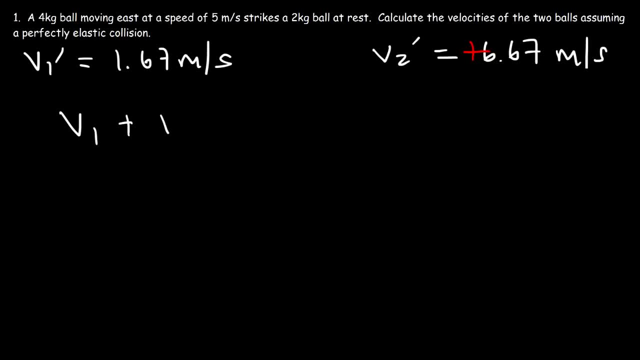 We're going to do it two ways. The most simplest way is to use this equation: V1 plus V1 prime Has to equal M1 V2 prime plus M2 V2 prime Has to equal V2 plus V2 prime. 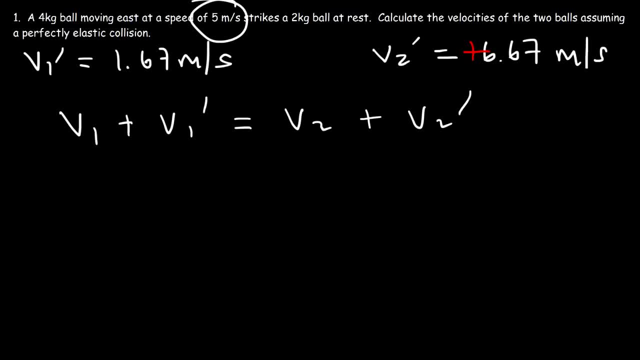 So V1, the initial velocity of the first ball is 5.. V1 prime is that value, that's 1.67.. The initial velocity of the second ball, because it was at rest, is 0.. And V2 prime is 6.67.. 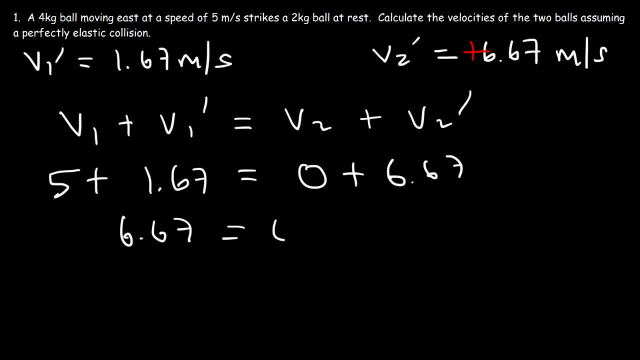 Now, 5 plus 1.67 is 6.67.. So kinetic energy is conserved. Now let's confirm it Using a more familiar equation. Let's use this one: The kinetic energy of the first object, the first ball, is 1 half M1 V1 squared. 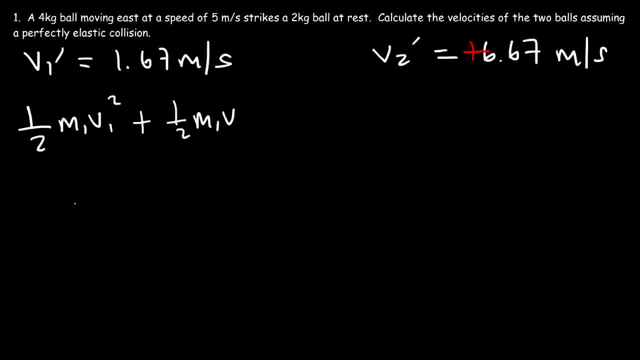 And the kinetic energy of the second ball is, well, that's supposed to be M2 V2 squared, And this is going to be equal to the final kinetic energy of the first ball, which is 1 half M1 V1 prime squared.